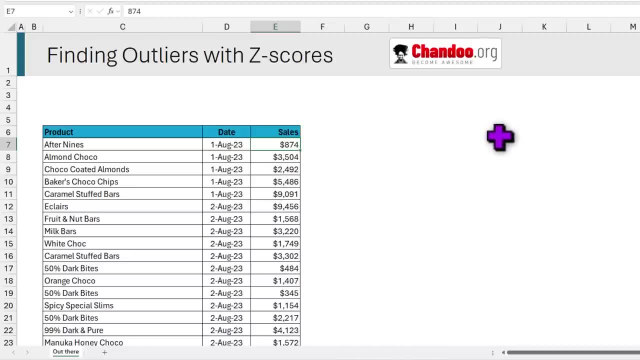 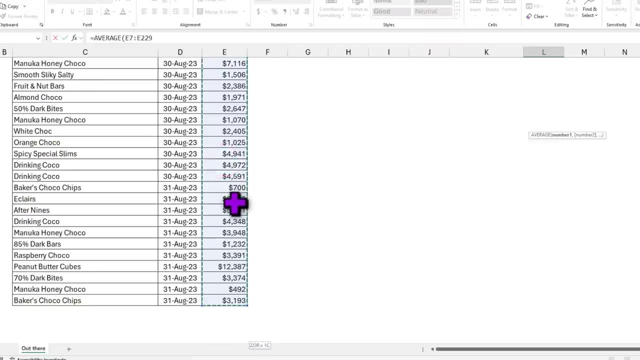 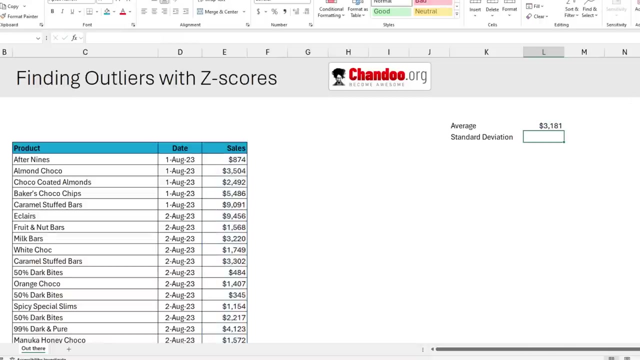 calculate the average and standard deviation of the data. I'm going to calculate them here. So let's set up a cell for average and one for standard deviation. Average of our sales data is average or average. So I'm going to grab all the 223 records and that works out to be $3181.. To calculate the standard, 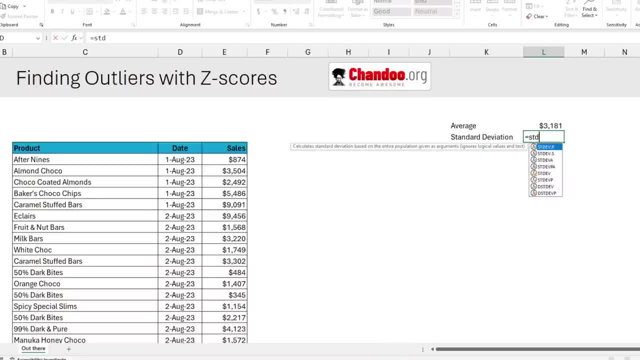 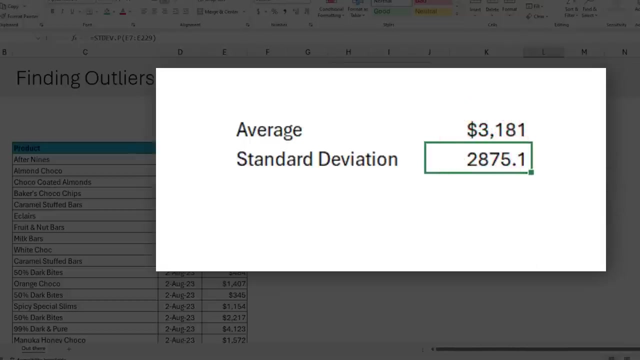 deviation, we can use stdevp function. You can see that Excel has many other standard deviation functions. As this is the entire data and not a sample, we are going to use stdevp function and select all the numbers again. The average is $3181 and standard deviation is $2875. 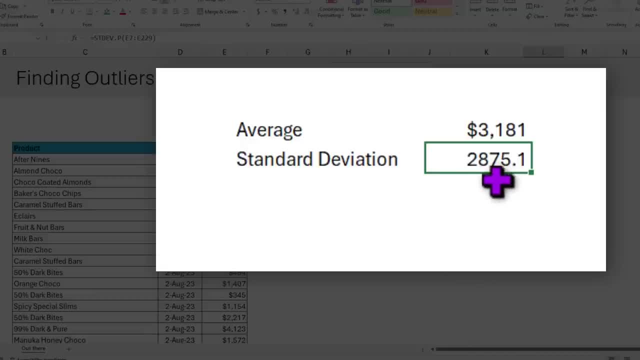 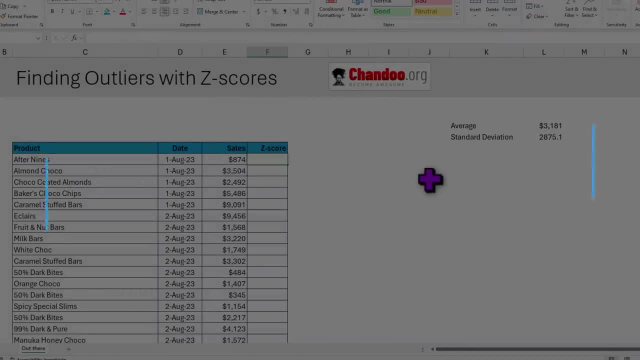 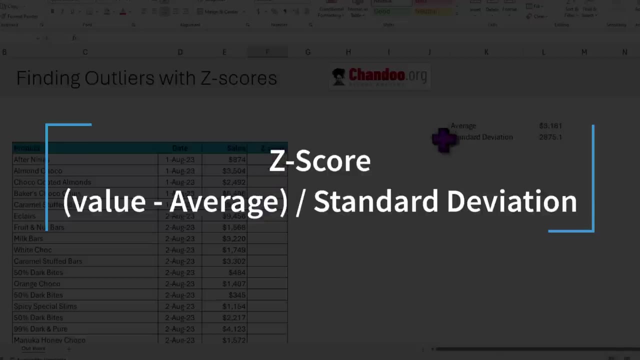 As you can see, standard deviation tells me that our data is quite varied. Now let's go ahead and calculate the z-score for each of the data points. Z-score for any value is defined as that value minus average divided by standard deviation. So we can do it like this: 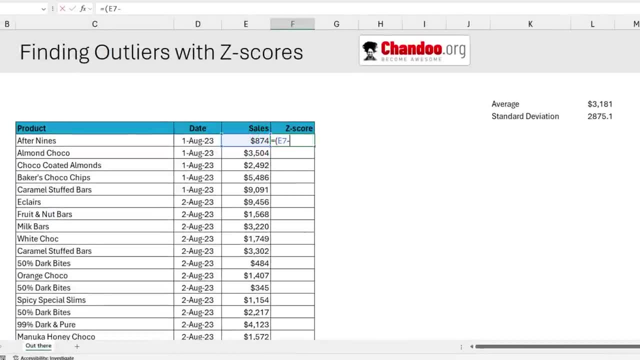 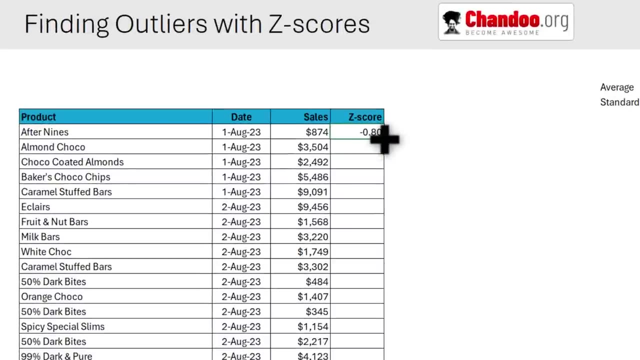 Open bracket. This cell value Minus the average here in L4.. I'm going to make it absolute Divide that with the standard deviation L5.. Once that formula is entered in one cell, you can just drag this down or click in the corner. 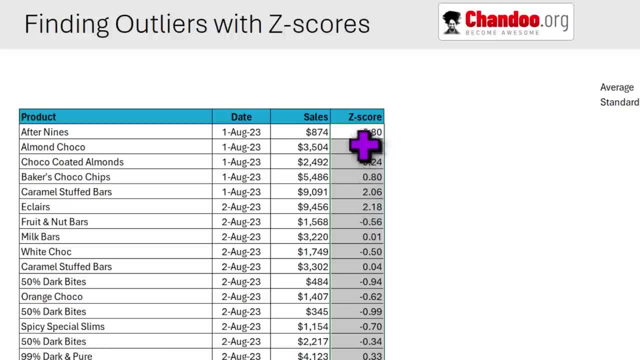 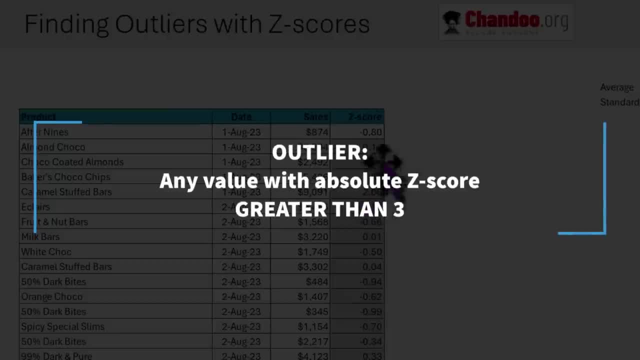 here to fill the g-scores down for the entire data set. Now that we have calculated this, we can identify outliers. An outlier is usually any data point that has an absolute z-score, So we can say that we have a z-score higher than 3.. 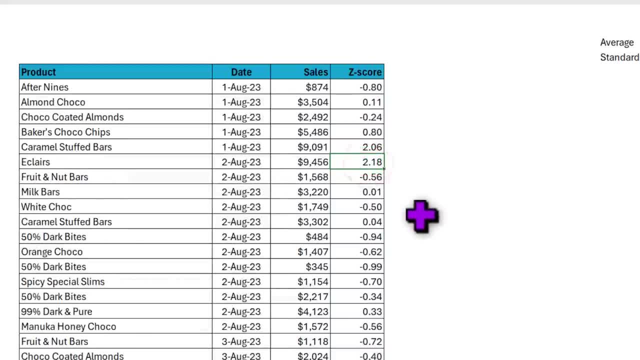 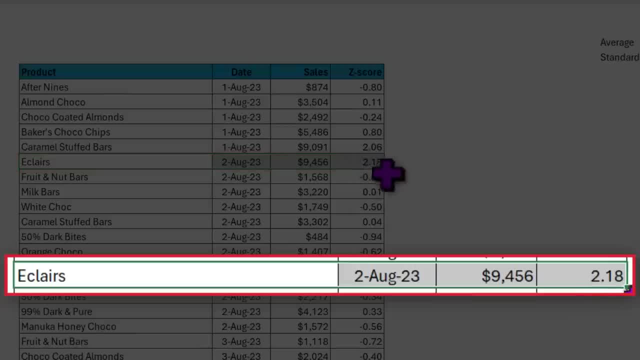 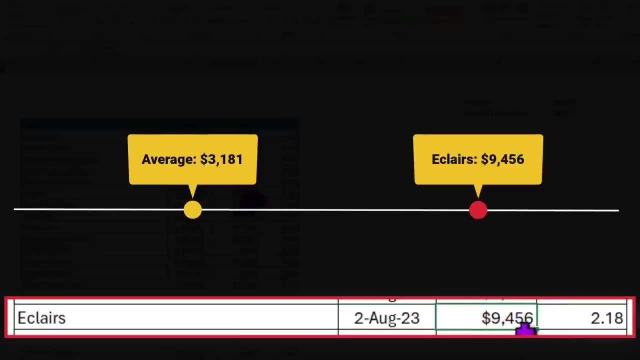 So here you can see that many data points have 2.18 here, which means this data point is 2.18 standard deviations away from the average cell value. So average is $3181 and this number, 9456, is 2.18 times away from the average in standard deviations. So usually we consider anything. 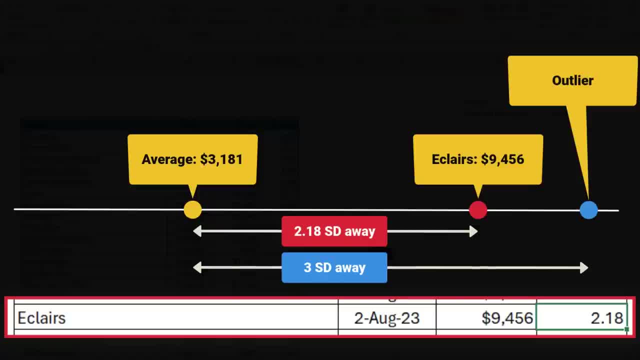 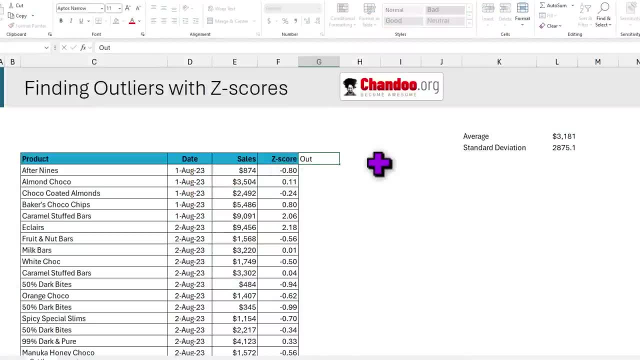 beyond 3 standard deviations away from the average as an outlier in normal data. So I'm going to add one more column here and then say outlier question mark And here we can simply say: if absolute value of my z-score is greater than three. 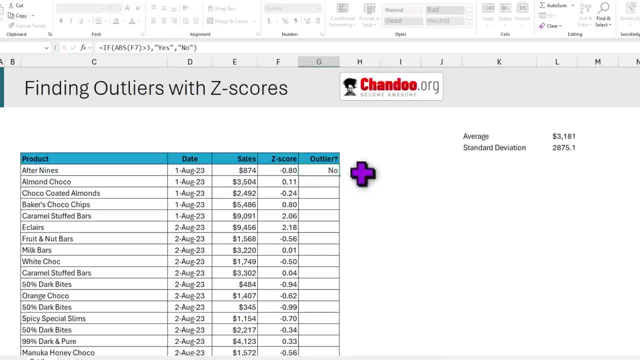 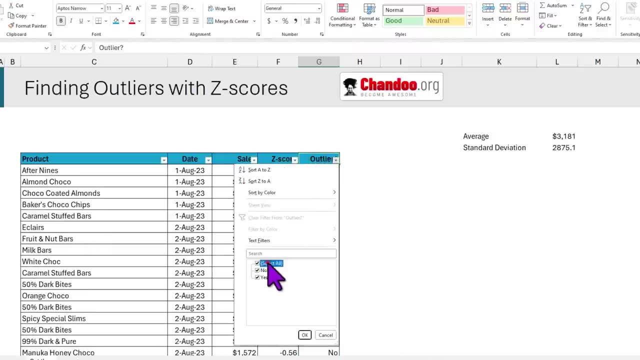 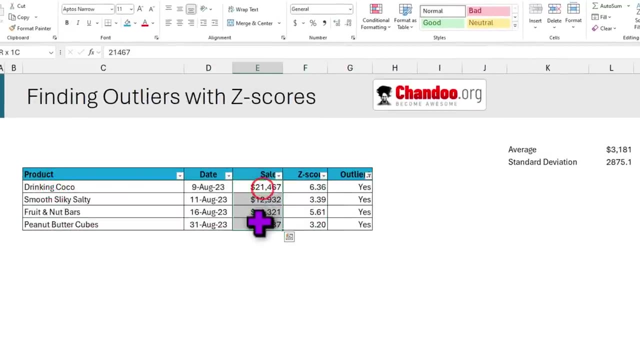 yes, Else no, And then you can fill this down. There will be some outlier somewhere. Let's filter those down to see what they are. so i'm going to apply filters and select all the yeses for my outliers and we can see that there are four records where the numbers are quite large to be. 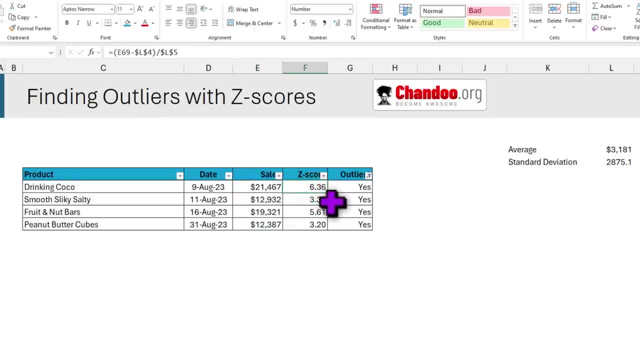 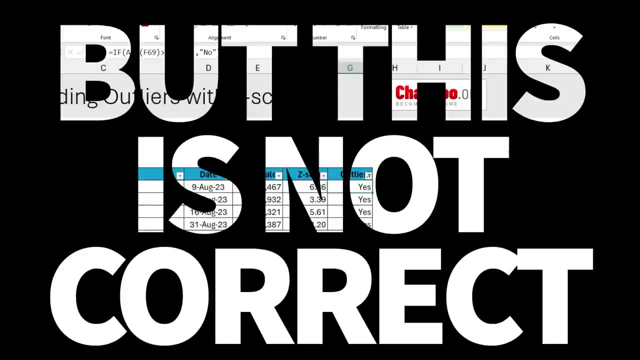 honest and they have very high z score. so here, drinking cocoa 21 000 and it is 6.36 z score. definitely an outlier, but this way of identifying outliers is not perfect, as we can have different sales for each product. identifying an outlier within all the sales of drinking cocoa would be. 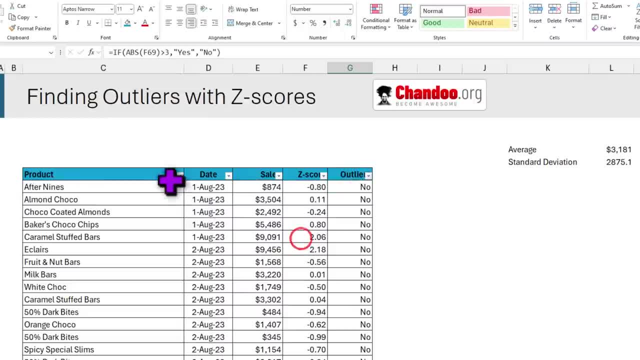 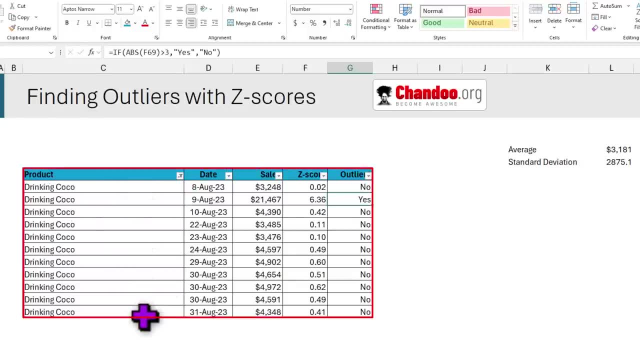 a better option. by that, what i mean is: let's clear out this and filter down for one of the products. so we have got all these records for drinking cocoa and you can see that this is how those values are. if i can identify what is an outlier within the drinking cocoa values itself, then it 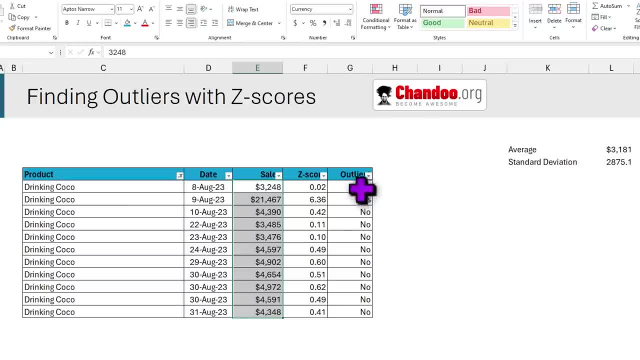 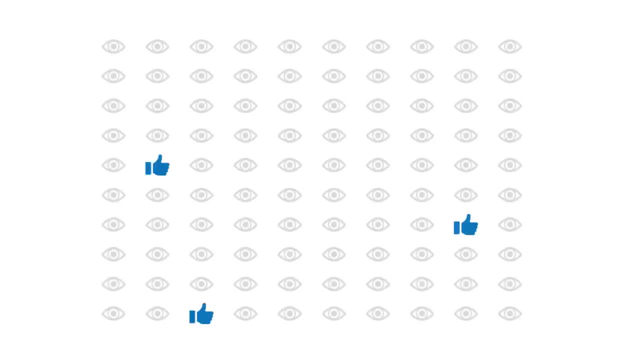 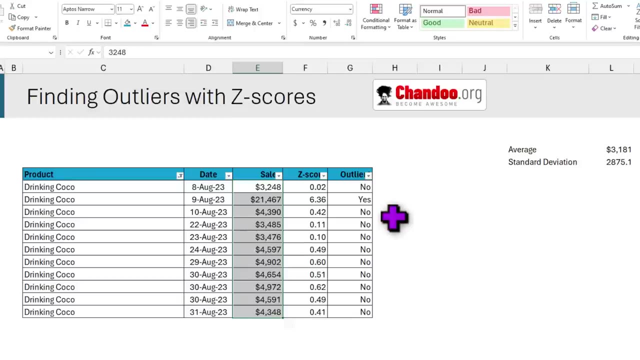 will be more meaningful, and we can do that quite easily with excel formulas. talking about all these outliers reminds me that just three out of every hundred people who watch my videos hit the like button, so that makes those of you who hit the like button an outlier or a really special person. so i want you. 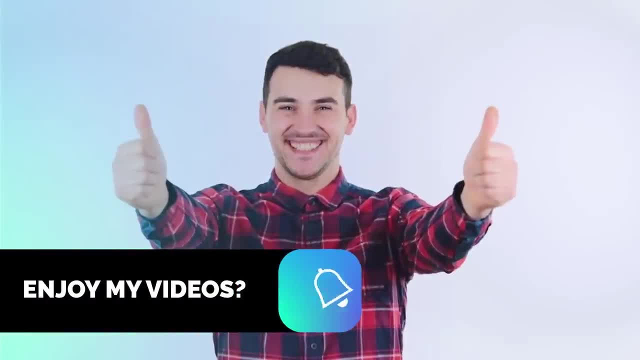 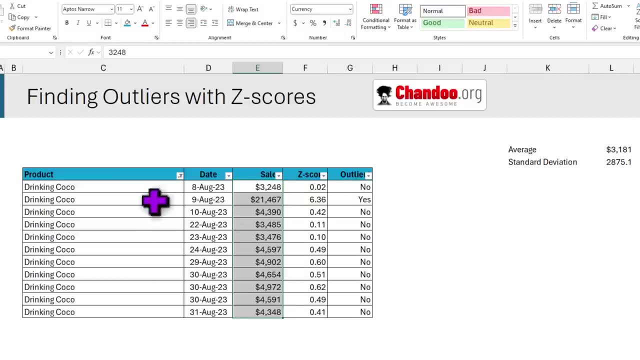 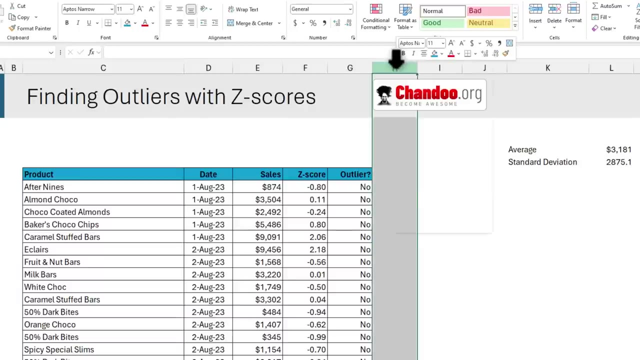 to become that special person. hit that like button and, if you have not already subscribed to the channel, consider subscribing for more awesome videos like this. now let's understand how to make z score, keeping the product in consideration. i'm going to insert a few more columns here just to make space for that, and in the first, 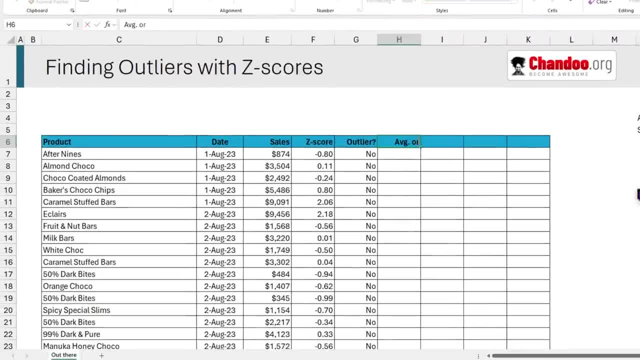 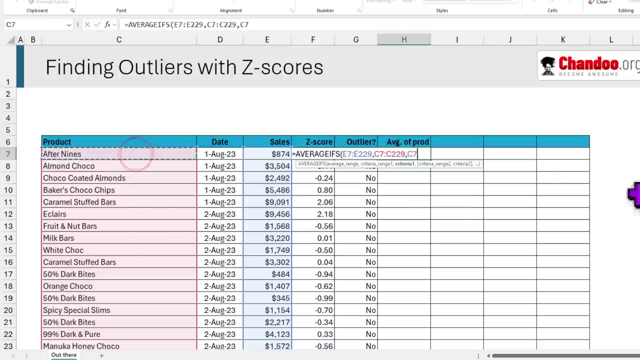 column. i want to calculate average of product. this is average ifs of my sales value. where my product value is average of product gets shown. so if you have a product in r and you have product number average, average, average and you have change in your sum, that'll mean you have change in. 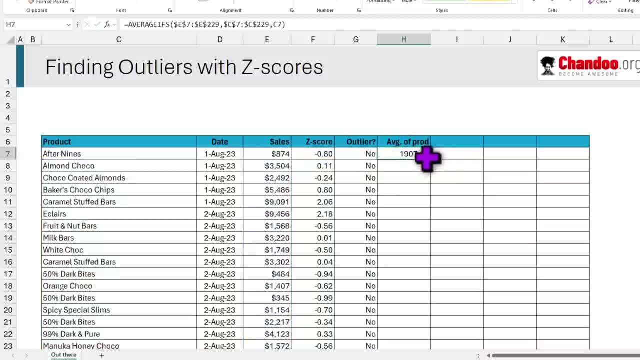 your sum. that rules the overall sales value. i'm going to write here how many trade in the market and i'm not going to be able to write this in the actual market, so i'm going to write f9, which is the number of products after nine, and i'm going to write these in. 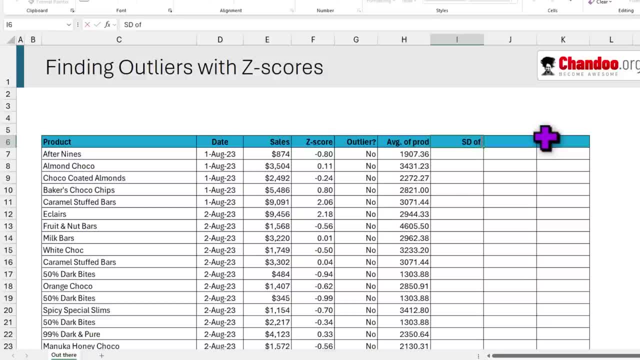 cells c7. now i'm going to select all of these bits. hit f4 to make them all absolute reference. Same for standard deviation of product. Now, unlike averageifs in excel, we don't have a standard deviation ifs function. We only have standard deviation. 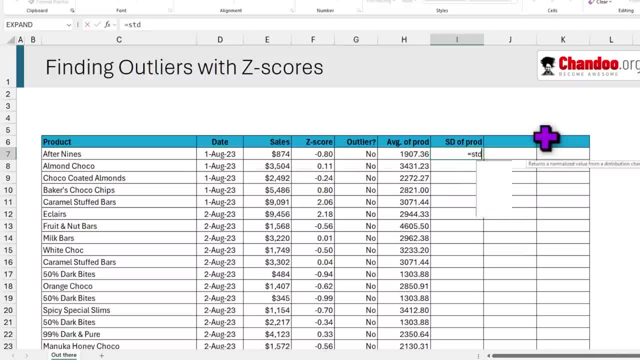 So we are going to use standard deviation, dot, p function and instead of giving all the data, we are then going to use the filter function inside. If you don't have filter and excel 365 to use it, I'll put a different formula in the 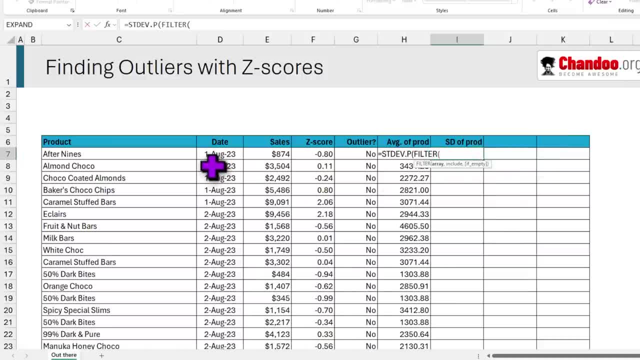 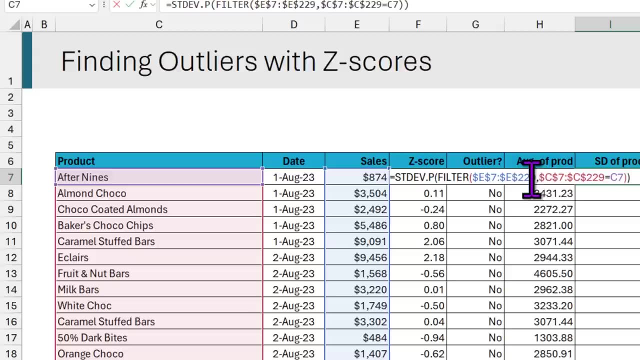 video description. that will work here. So filter, and then here we are just going to pick all the data again, and the filter criteria is: product name is equal to this. So notice the structure of this filter. it is similar to how our averageifs, is only difference. 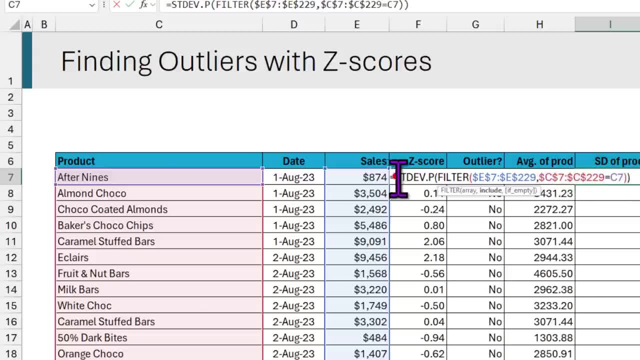 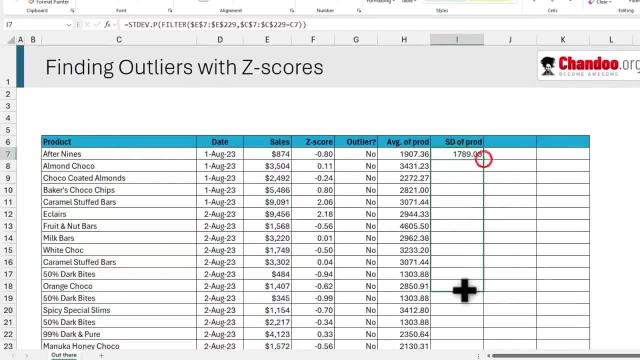 is here. we are just saying equal to and then putting the product. So when you write this formula and hit enter, you'll get the standard deviation just for after 9.. And when you again drag this down, you'll see different numbers. So, for example, almond choco, despite having a higher average, has similar standard deviation. 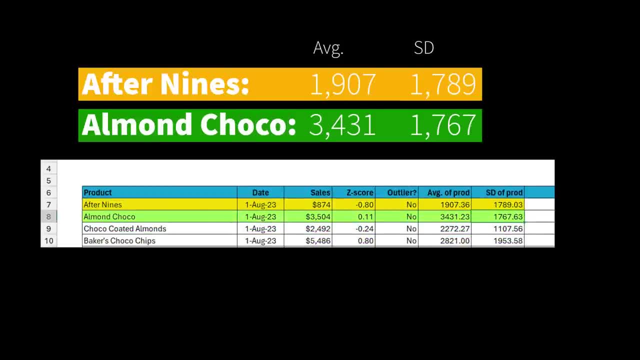 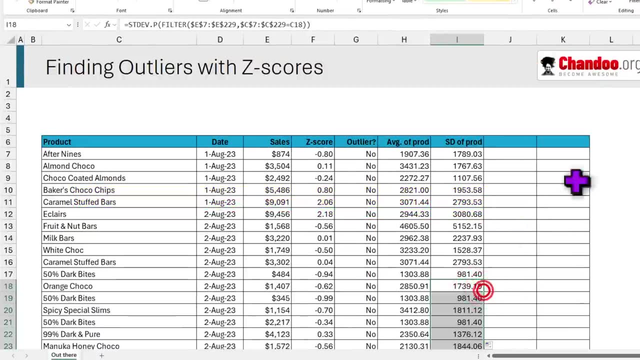 to after 9s, indicating that the sales of almond choco are less varied than sales of after 9s. Let's fill this down as well. and now let's calculate the z score at product level. Here the formula is The value minus corresponding average divided by standard deviation, and you can fill this: 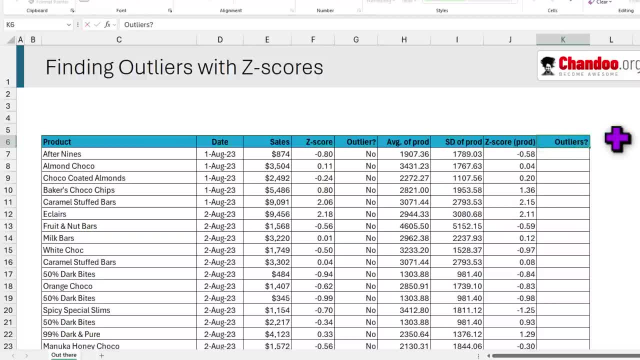 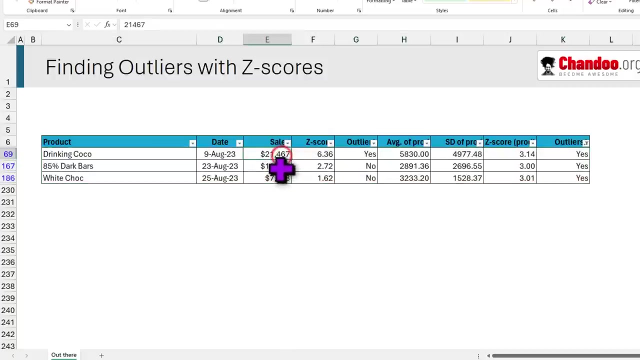 down and now we can identify outliers again If this value, absolute of this value, is greater than 3, yes, no. and now let's see what are the outliers according to this new definition. So we are now finding a different set of numbers. If you remember, earlier we had the same values, but the 7001 is not there. but now we are finding. 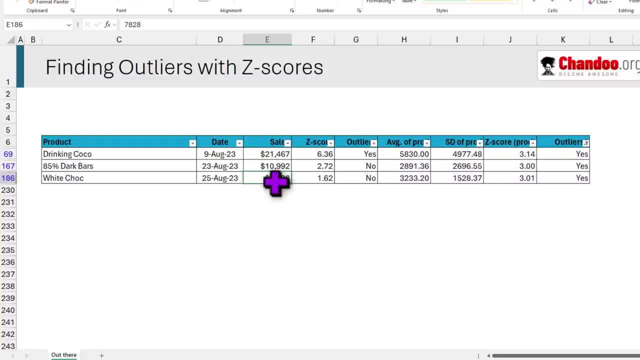 that the white chocolate value of 7800 is actually an outlier, even though it wasn't an outlier as per the original criteria. So here these two were actually. no, even the 85% dark bars. here the drinking cocoa was clearly An outlier in both cases. so in the original all average and all standard deviation. it. 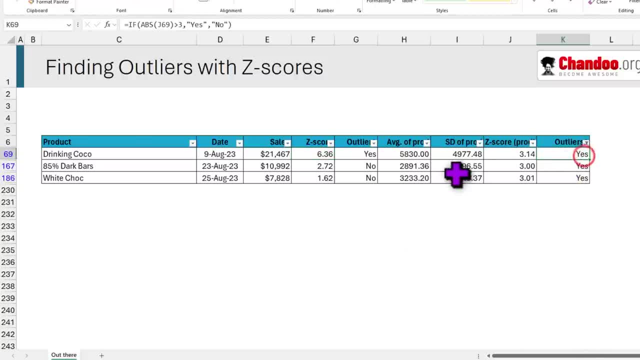 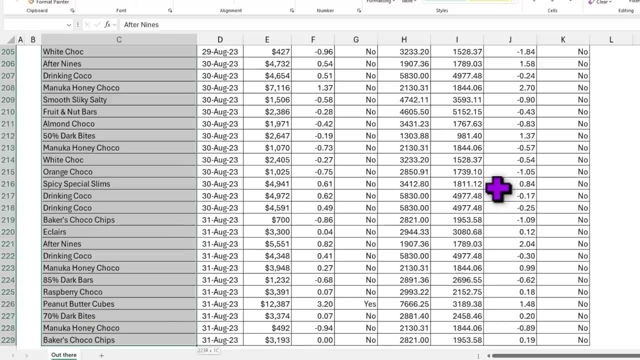 has 6.36 z score, whereas at a product specific level, it has 3.14 z score. Let's put the cherry on top of all of this: we can select all of this data and then use conditional formatting to highlight the rows or the records that have these outliers. 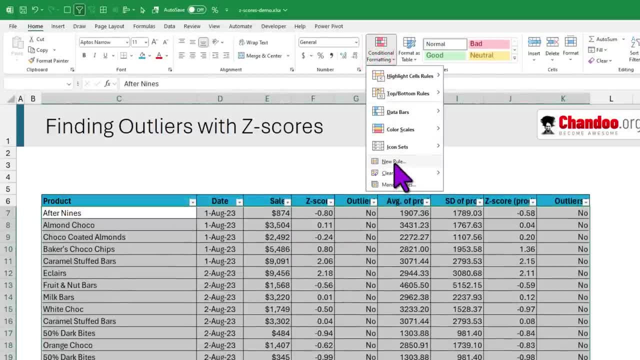 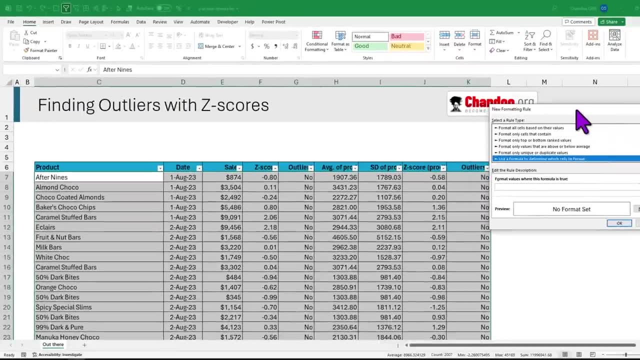 So once you select that, you can go to conditional formatting, Create a new rule, And this rule is: we are going to use a formula. the formula would be: you can just look into the outlier column, or let's just say you don't have that and you only have z score column. 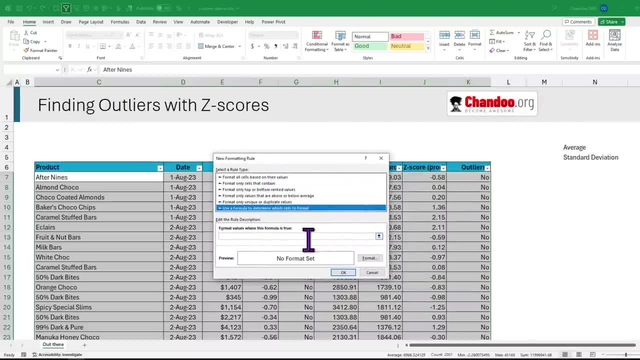 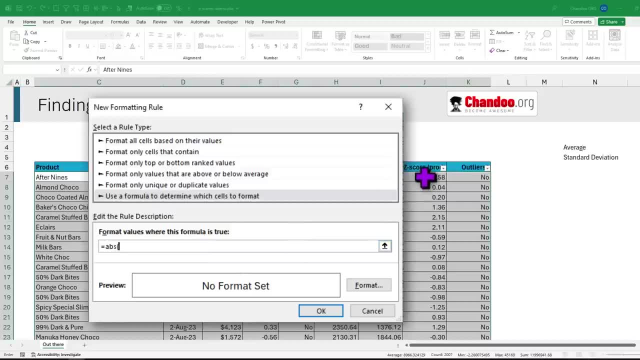 you can also write the rule there. I'm going to use the z score column to write the rule, so here the rule is equal to absolute of- and then select the z score column value here in my data it is in j7. I'm going to change. 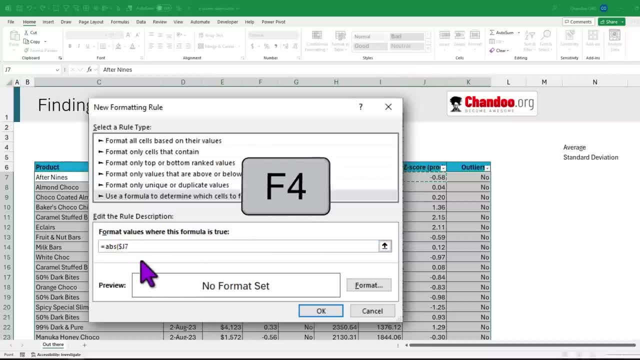 the nature of this reference, By hitting the f4 key a couple of times- to dollar j7. it locks the column to j but keeps the row number relative. so every row it checks the corresponding column: j value. so absolute of dollar j7 greater than 3. so that is my condition and then I want to format this in: 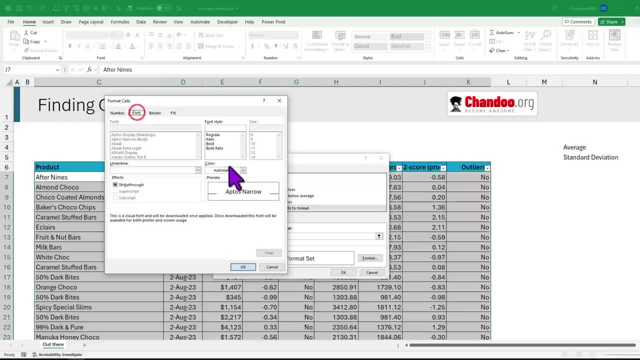 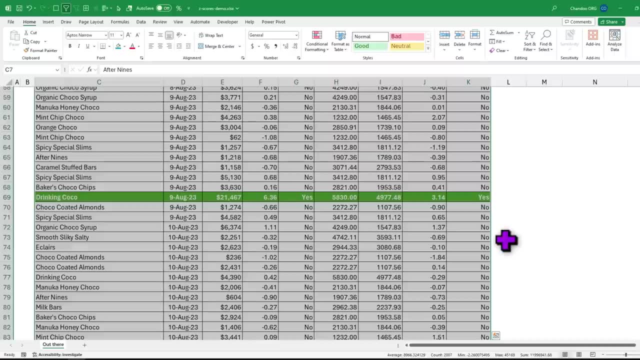 a bright color like this and change the font color to white and make it bold. Once You know It's okay, any outliers in your data will be immediately highlighted in a really striking font and color like this so we can immediately spot those values. 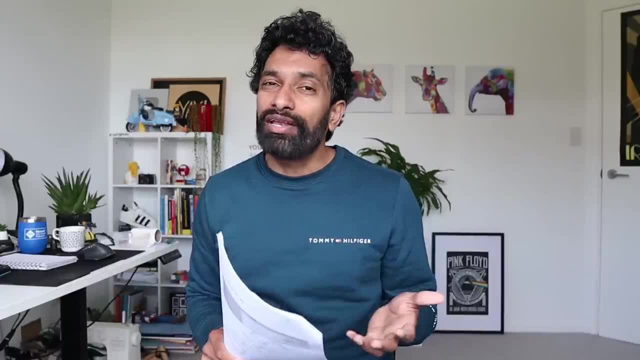 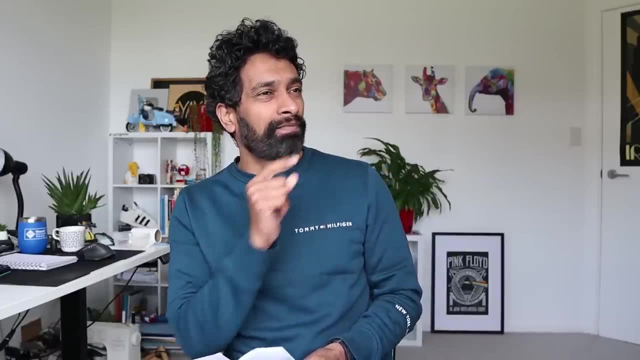 Now do you know that, given monthly sales data like this, we can use excel to predict the future sales, and it's really easy to? here is a video that talks about that. click on it, go, and before you go, make sure you like this video as well and subscribe to the channel. if you enjoy my content, I'll catch you there. Bye.